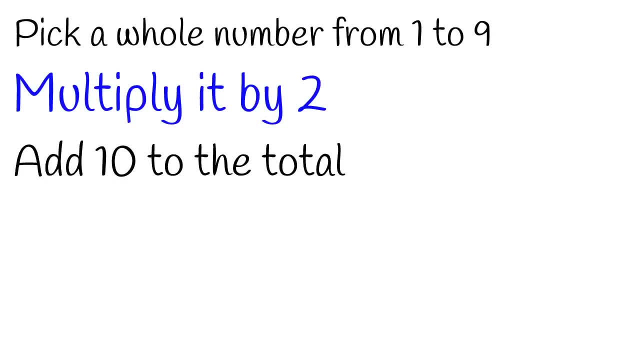 the total. Ok, So next, add 10 to the total. Ok, So next, add 10 to the total. Ok, So next. Now you have to divide this number by two. Now, from this number, subtract from the number that you picked. 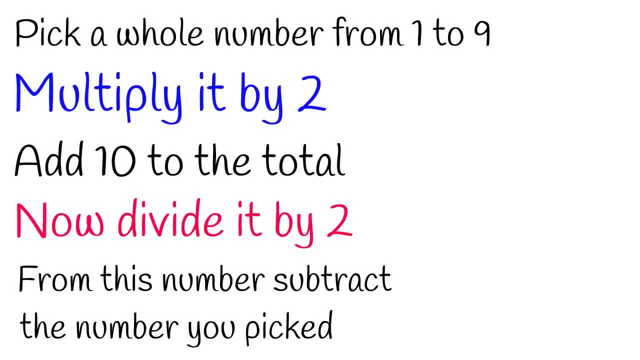 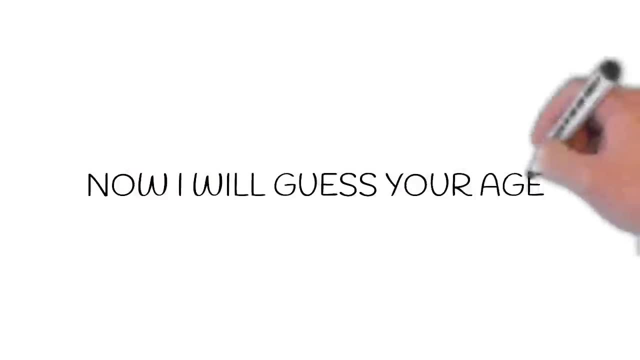 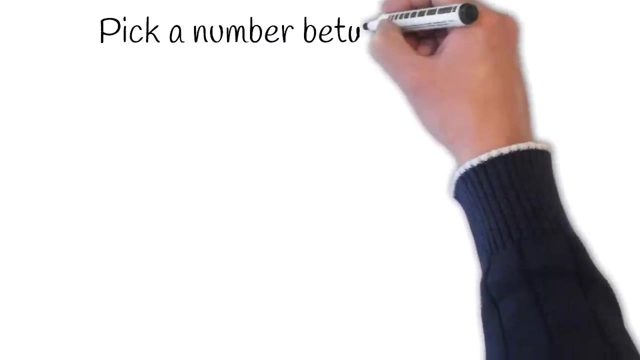 Yes, the whole number that you have picked. You have to subtract this from your total and tadadaaa, your answer is 5.. Am I correct? Okay, so for the next trick, I will guess your age. So first pick a number between 2 and 9.. 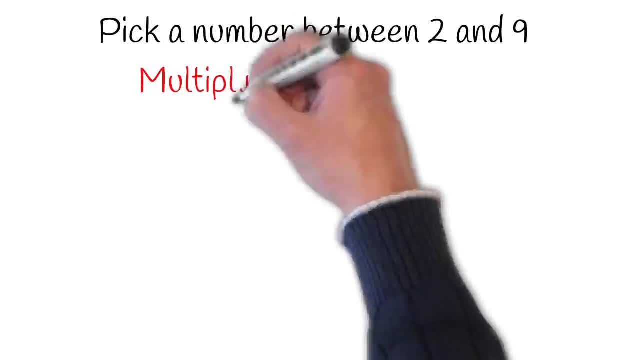 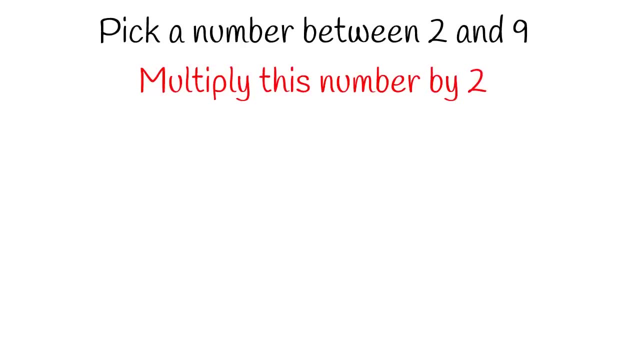 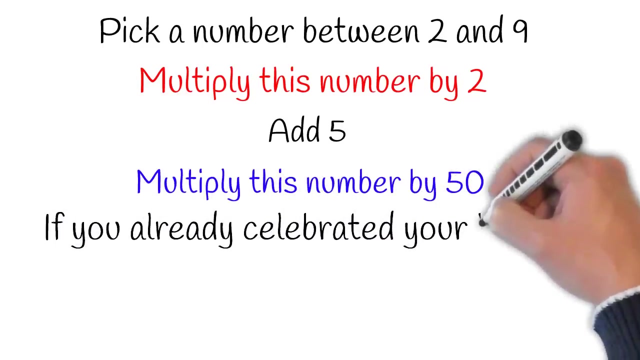 It can be any whole number between 2 and 9.. Now multiply this number by 2.. Done Okay. Now add 5 to it. Now multiply your answer with 50.. So if you have already celebrated your birthday this year, 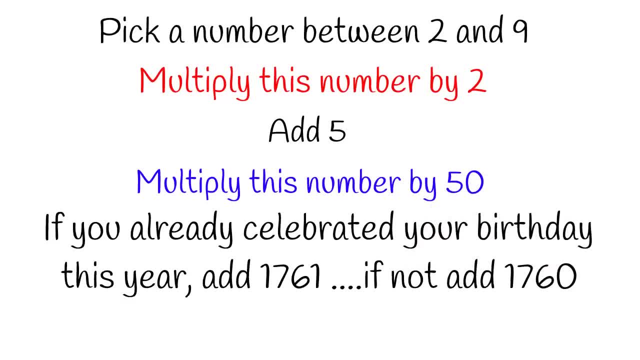 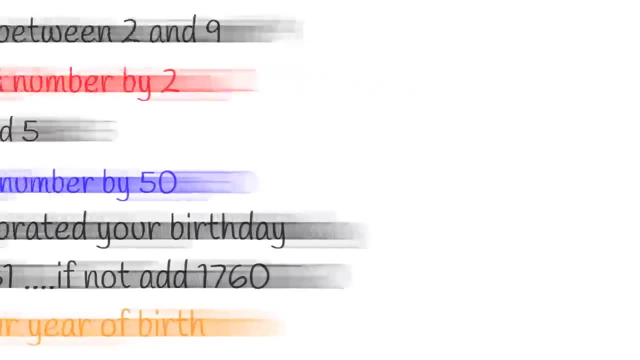 then add 1761.. That is 1000.. Add 1761 to your answer. If you have not celebrated, then add 1760.. Then subtract your year of birth from your answer. Okay, so let the magic reveal itself. 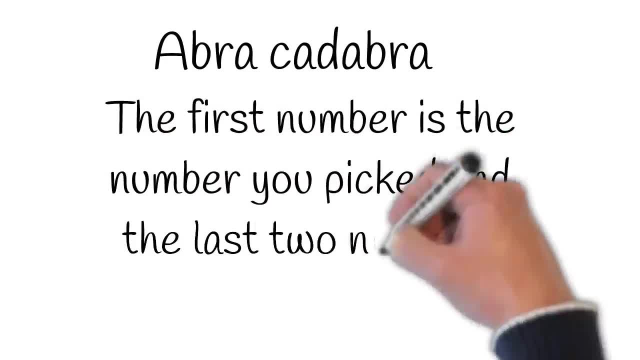 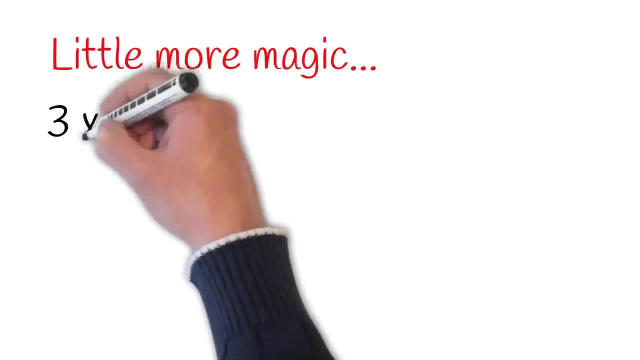 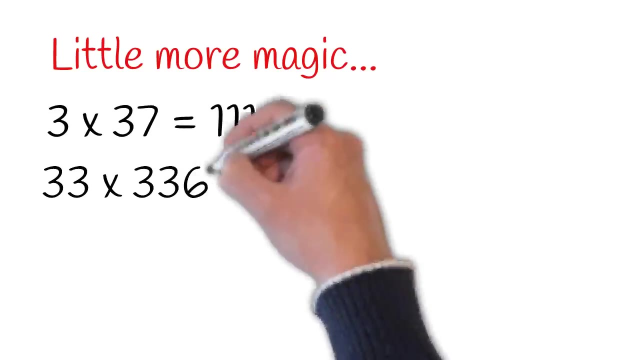 Let's say Abra Kadabra. So in your answer the first number is the number you picked and the last two numbers are your age, Am I correct? So there are few more interesting simple magic of multiplications. So 3 into 37 is equal to 111..